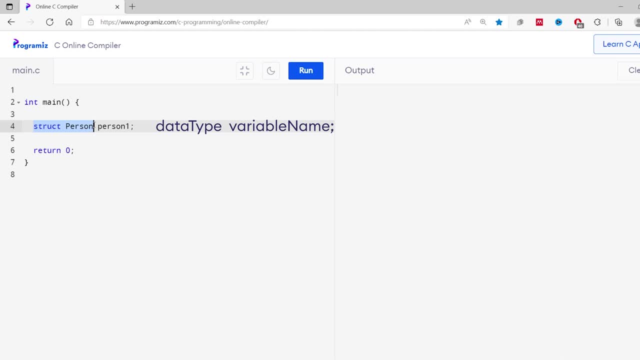 regular variables. So let's create a variable of struct person type. So let's create a variable where struct person represents data type and this person one represents the variable name. Now we can use these struct variables to access the members of struct. Now I'll add here person one. 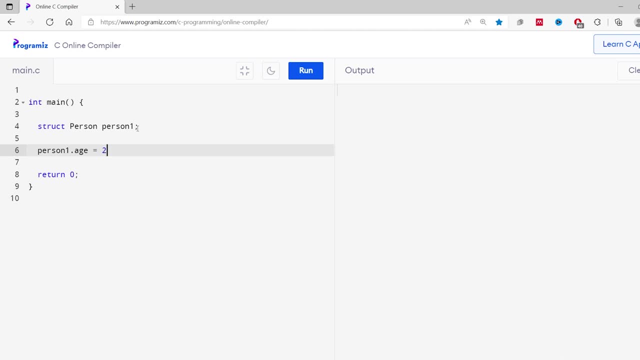 dot is is equals to 25 and person one dot salary is equals to 4,321.78.. Here I have used dot operator to initialize the struct. members is with the value 25 and salary with the value 4,321.78 for the person one variable. Now let's print the value I'll use. 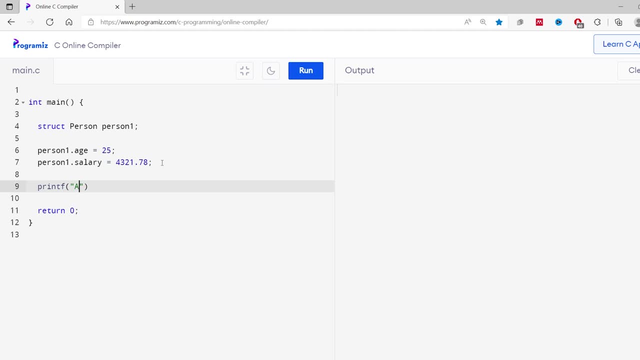 printf statement Here is of person one is percent dn comma person one dot is. and another print statement that prints the salary of person one that is in double, So 0.2 lf comma- person one dot salary. Similarly, the same dot operator is used to access. 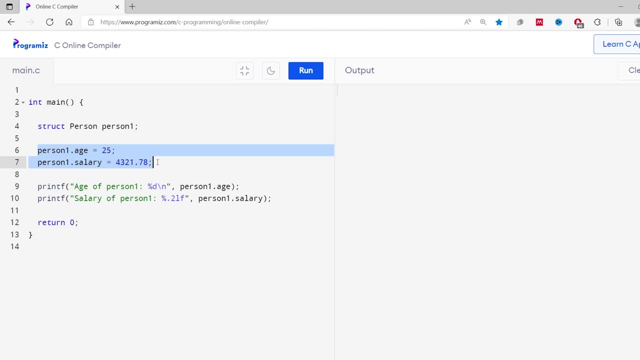 the value of struct members is and salary for the person, one variable. Now I'll complete this program. Here I'll add include stdio dot h and add here: struct person curly braces. double, sorry, double. salary and int is. Now I'll run this code. 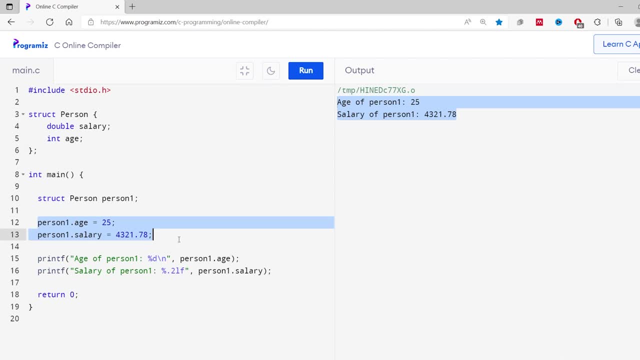 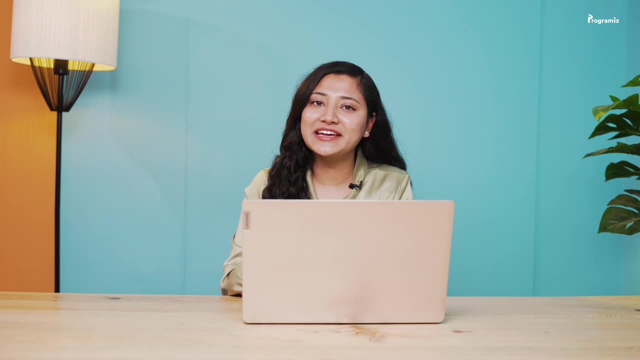 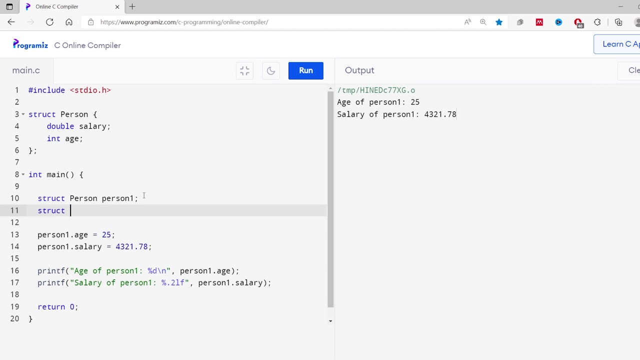 Here you can see we have successfully initialized and accessed the struct members for the person one variable. In this view, we can create as many struct variables as we want and all stock members can use the as and salary members of the struct. Let me show you inside the main. I'll add here: struct person, person two. 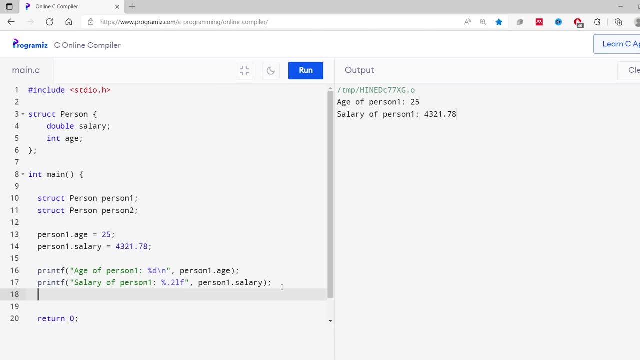 structormける PRSZN. eating simplesmente the stock members for person to variable as well. so I'll initialize: person to variable is equals to 31. person to dot salary is equals to 70 thousand nine hundred forty three point two, and I'll print this, so is of person to call them. 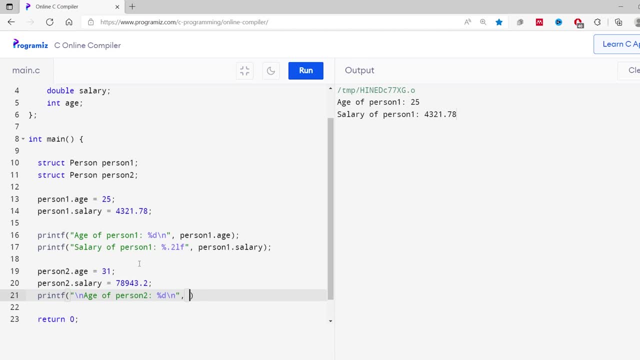 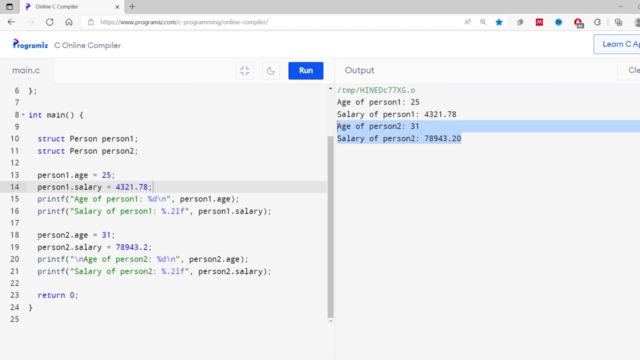 percent D comma person to dot is. and print F salary of person to percent. point to LF comma person to dot salary. so I need to move this space from here. now let me run this code. you can see we have successfully used the stock per person to as well, by the way, do you want to? 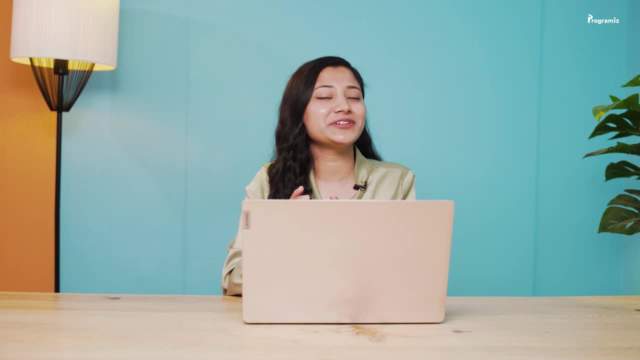 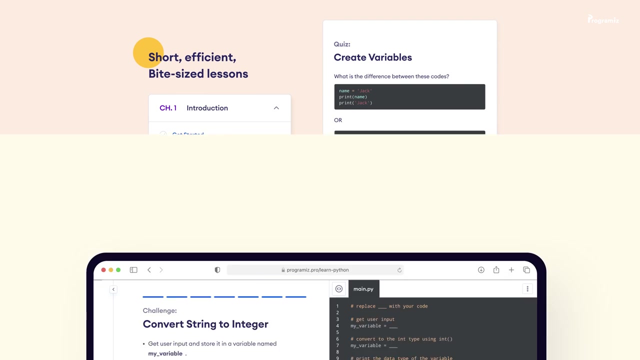 take your programming journey to the next level. watching tutorials is fine, but it has one limitation: it's hard to learn and practice together at the same time. lucky for you, we recently launched program is pro that provides tutorials along with quizzes and challenges, which will help you practice and test your 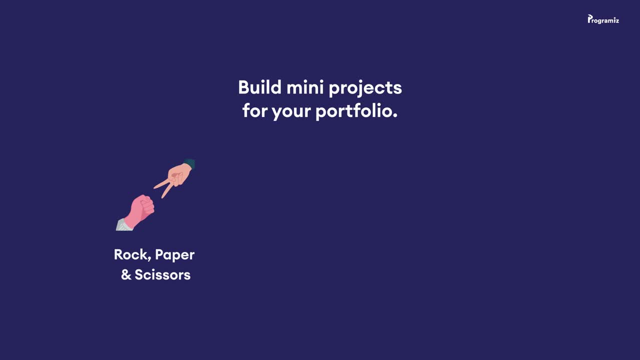 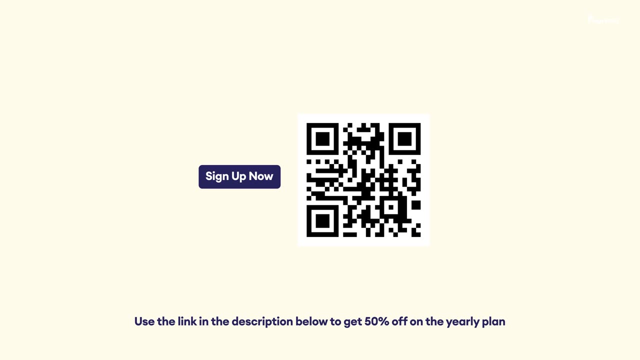 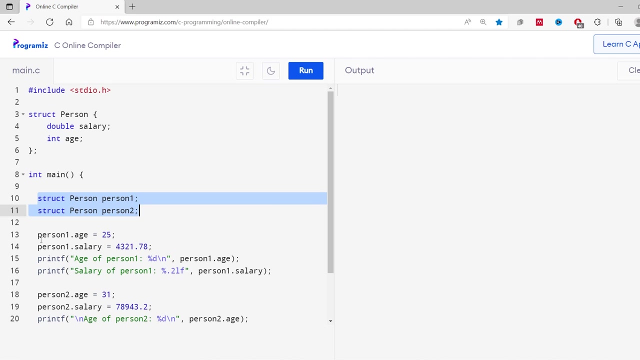 learning in real time. also, the course includes projects to give you an experience of how programming works in the real world. sign up now. visit the link, which is also available in the video description below. in this example, we are creating the strop variables in one line and assigning 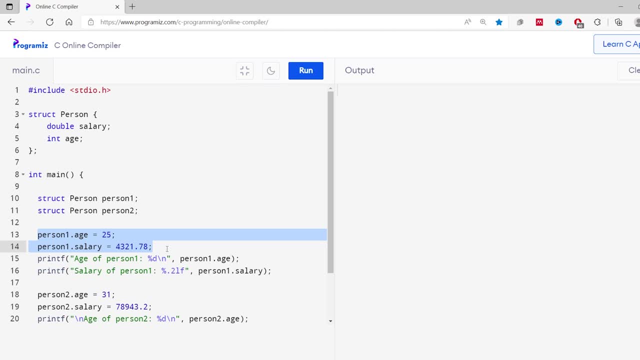 member variable in another line. instead, we can simply create the strop variables and initialize members in the same line. let me show you. I'll remove this part of code. so remove this part as well, and remove these two lines of code, and so I'll simply write here: 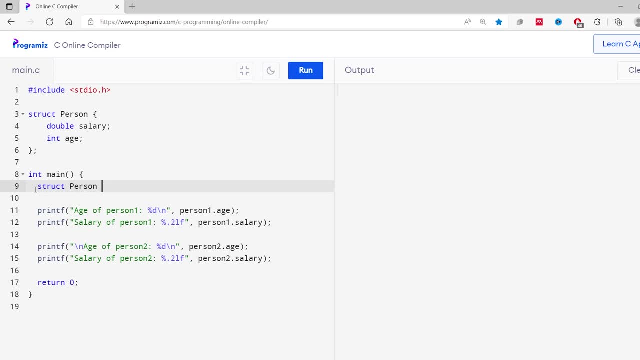 the strop Hear Weľ. Now, here we will get the next principle. here we will call theb strop strop person. person1 is equals to curly. bracesas is equals to 25 comma. dot. salary is equals to 4321.78. 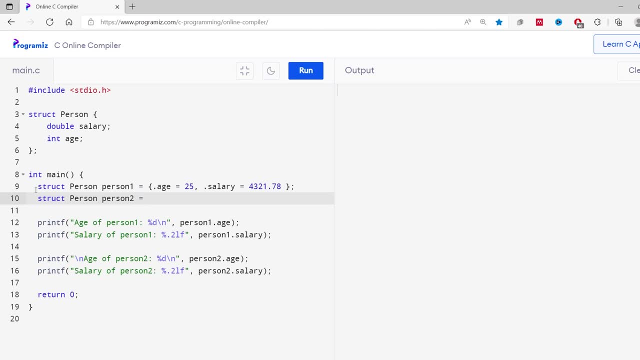 and I'll close this. Bun fell just and another strop person. person 2 is equals to curly braces. dot is is equals to 31 comma. dot. salary is equals to seventy eight thousand nine hundred forty three point two, and let's close this now. let me run this code here. you can see we get the desired output also. 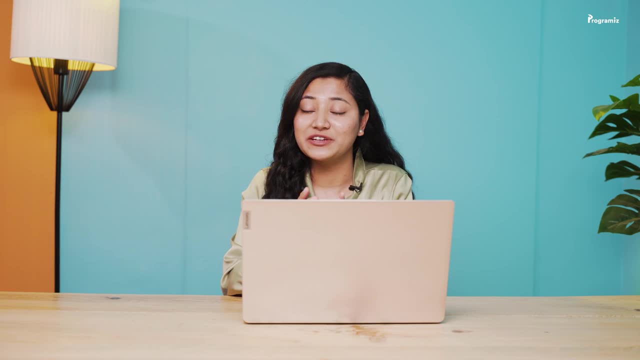 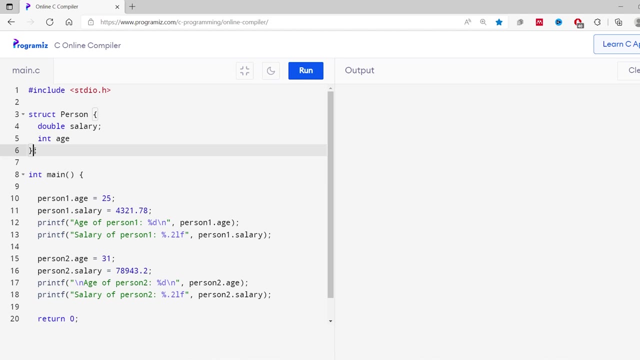 we can create struct variables while defining the struct. let me show you in this previous code I'll remove this part of code and here I'll add these struct variables: person one, comma, person two. now let me run this code. you can see we get the same output. 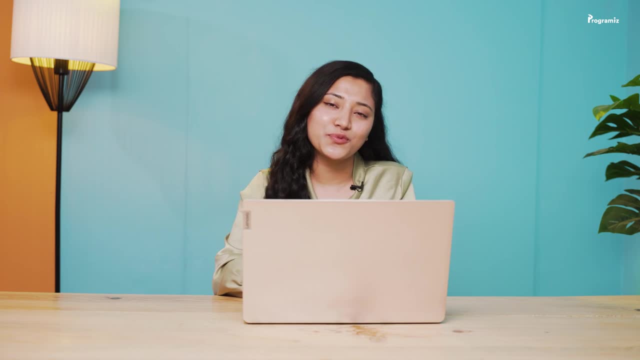 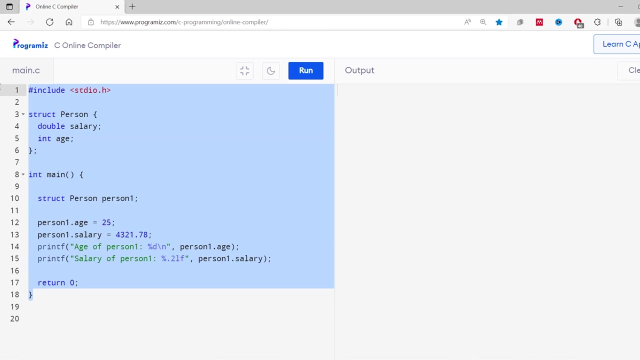 while creating the struct variables, we have to use both the struct keyword and the name of the struct, which is too long. instead, we can use an alias. the type def keyword allow us to use an alias for struct. let's see an example here. we have our code from our earlier example. in this case, instead of struct. 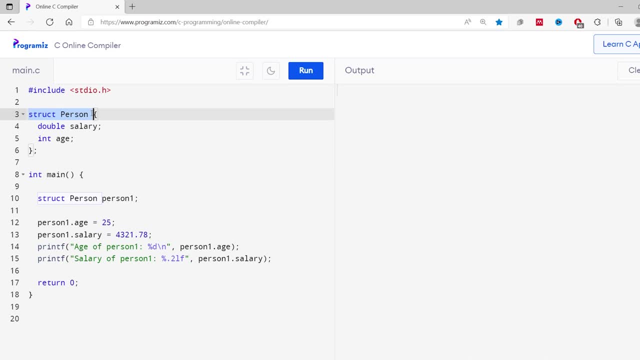 person. we can use an alias with the help of type def. let me modify this code here. I'll add here type def in the struct definition and person at the end. now this person can be used as an alias to struct, so we can now create a struct variable using person instead of struct person. so I'll remove. 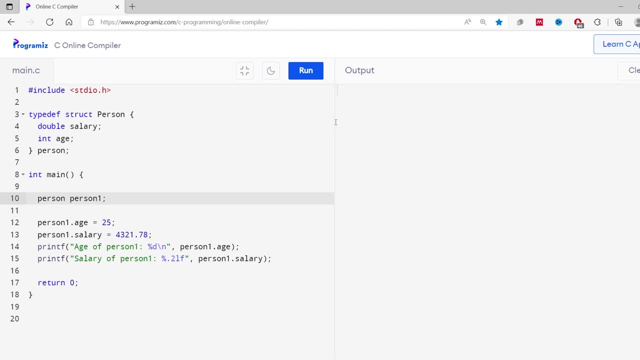 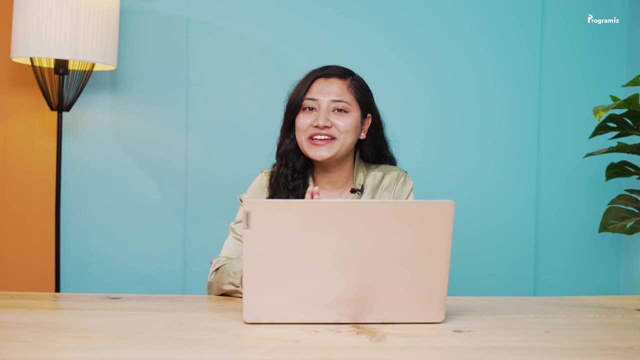 this and I'll write here. person. now let me run this code. as you can see, we get the desired output. okay, guys, we need your support to keep these types of content free for all users. YouTube really likes engagement on the videos, so leave a comment below, press that like button, hit subscribe if you haven't. 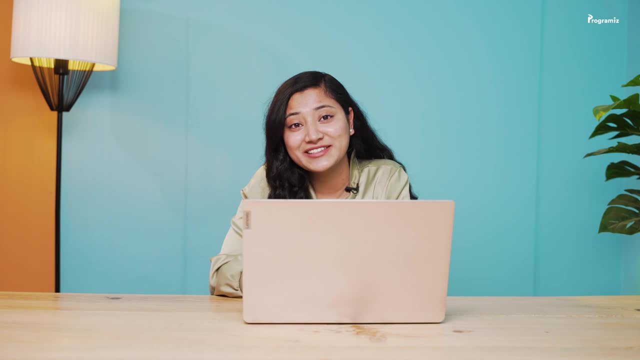 already. let's get the engagement score higher so that more people can discover and enjoy these courses. let's see one practical example of struct. we'll create a program to add two complex numbers. we know that a complex number has two part: real part and imaginary part. so while performing addition between two complex numbers, we 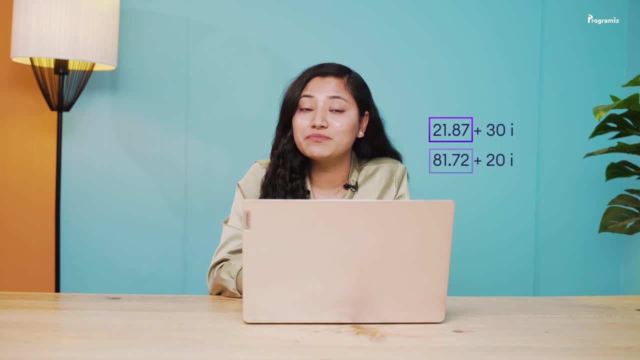 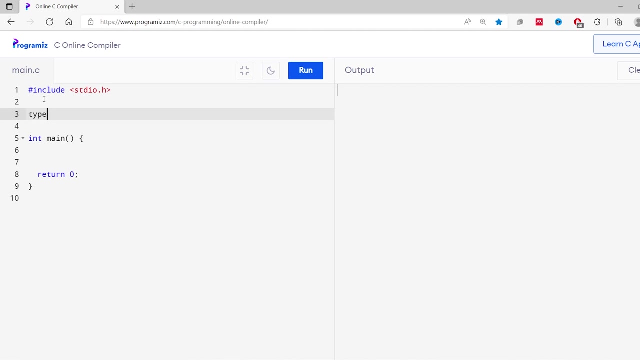 always add the real part of complex number with the real part of a complex number and the imaginary part of complex number to the imaginary part of second complex number. now you know the mechanism of the program. let's start writing code. first I'll create a struct, type, def, struct- complex and curly. 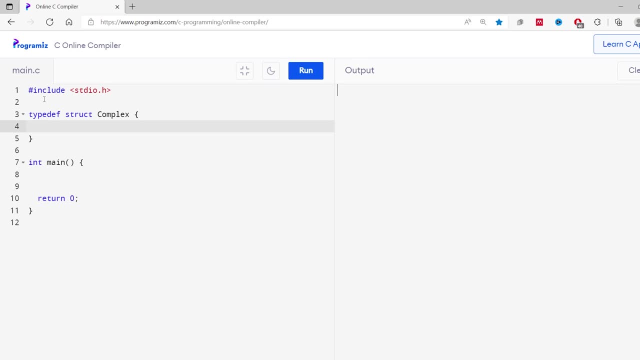 braces and it has members, real and imaginary. so double real and double imaginary. so I'll just write: imagine: so this represents the real and imaginary part of complex number, and we will add complex at the end of the struct. so complex here and semicolon. now let's create two complex variable. 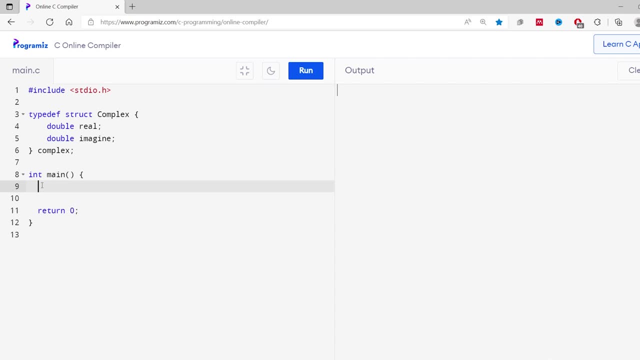 you can see that we have two complex variables. so we have two complex variables. so we have two complex variables. so we have two complex variables whose sum is to be found. so I'll write here: complex. c1 is equals to curly braces dot. real is equals to 21 point 87, and if imaginary value is, imagine is: 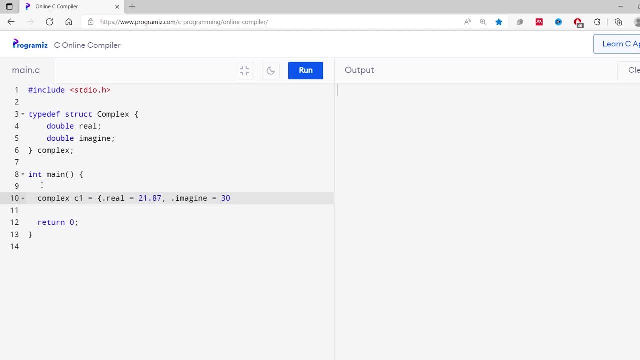 equals to 30, and then we'll close this. and another variable, complex c2, with value. real value is equals to 13, point 34, and imaginary value, dot imagine is equals to 112, point suppose this is 1 at 12, point 2, 3 and we'll close this. 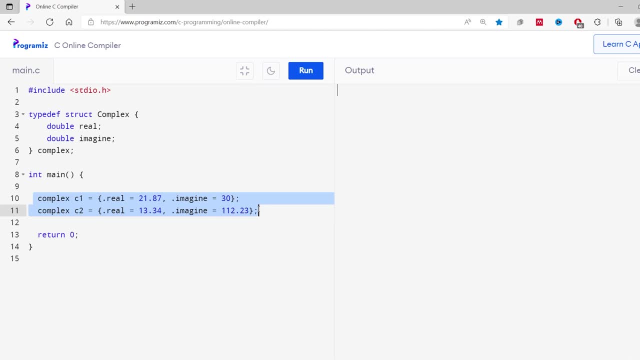 remember we are assigning value while creating the complex variables. now let's create a new complex variable and let's create a new complex variable and let's create another complex variable to store the sum of these two variables. so I create here complex sum, as mentioned earlier. let's add the real and the